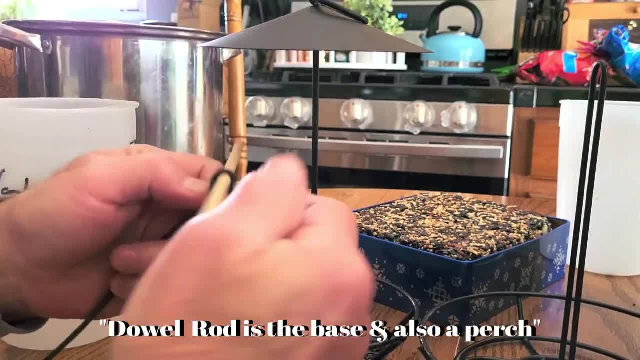 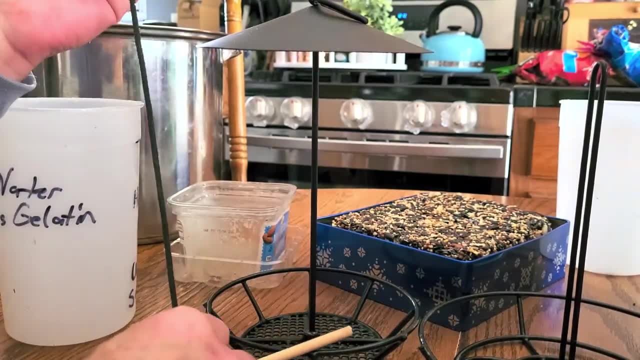 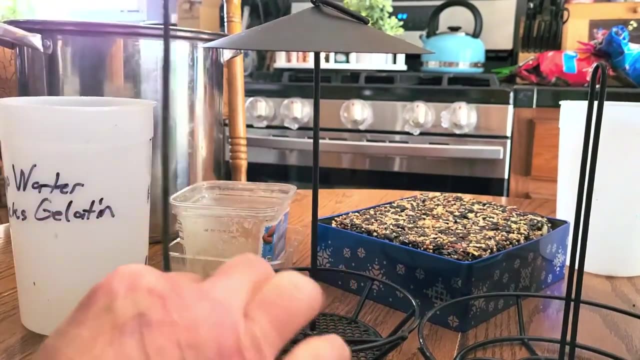 over and over, And then I just cut some quarter inch dowel rod So this Dacron goes through the center of the cake, the cylinder cake suet that we're going to make here pretty quick, And then you can just hang this from a tree and the suet cake fits right on here, And then you can just 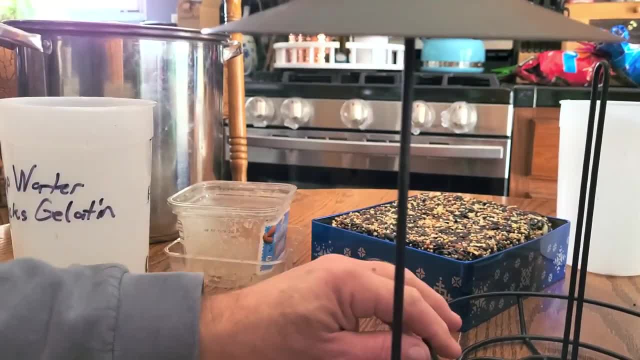 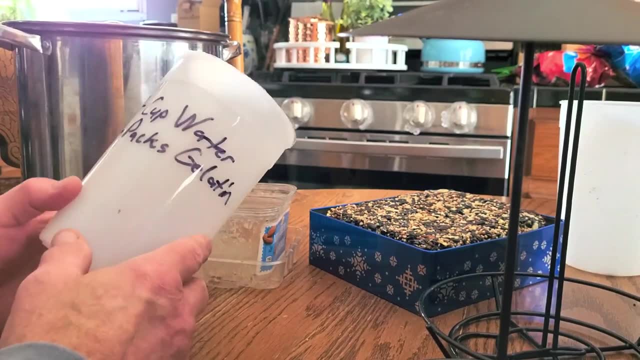 put it in here, the cylinder. So there's a lot of different ways you can put it, or you can actually just put it on top of a flat feeder or platform feeder. Anyway, our recipe, after trying and trying to get it quite right. this holds five cups of seed or five cups of water, pretty much. 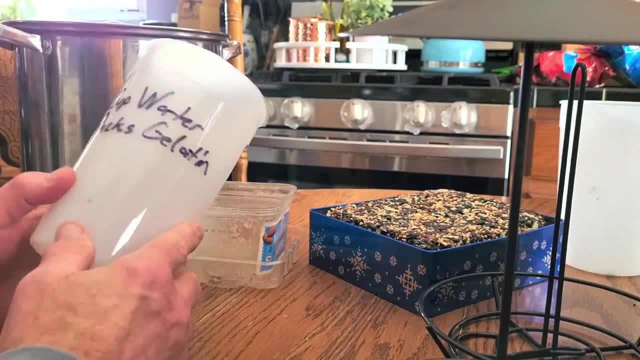 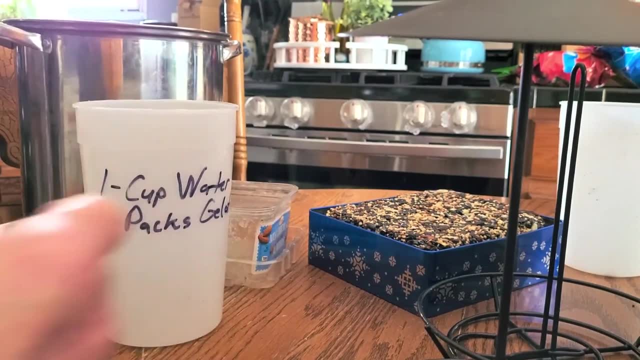 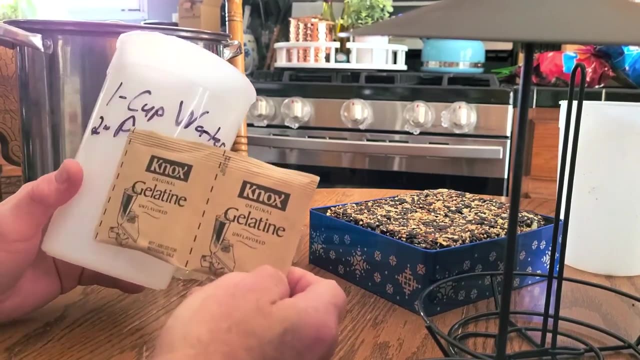 the same. The main ingredient is gelatin. What we found out is if you use one cup of water with two packs of gelatin. we've been using Knox. It's super cheap. You might be able to find it in bulk in cans or something, but it's averaging. 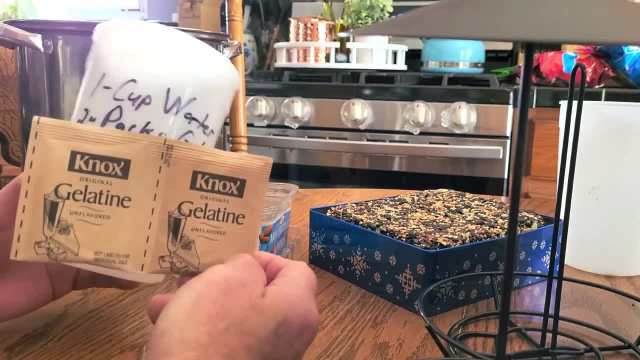 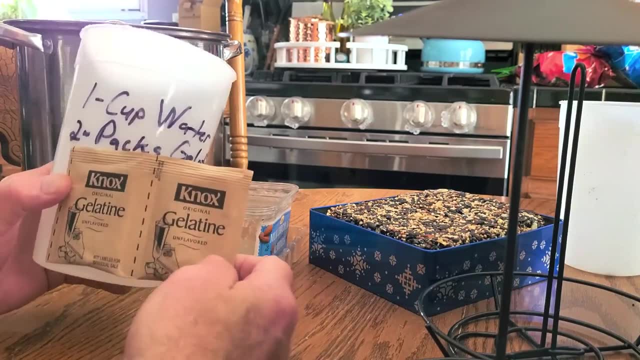 about 40 cents a pack. So to make one suet cake in this size is going to cost us, with some miscellaneous seed on top, probably a little, you know, maybe a buck 20 per seed log. So the ingredients is you. 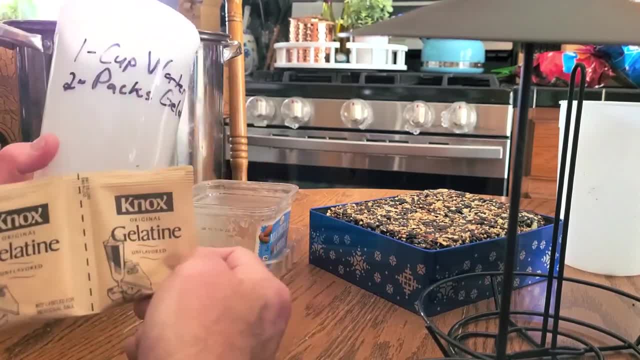 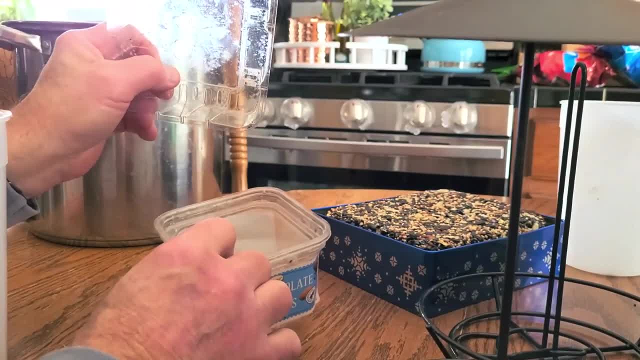 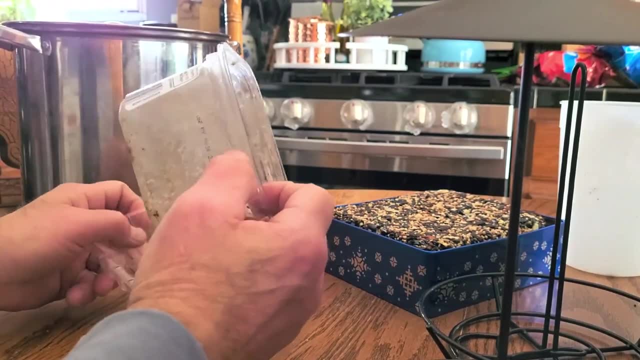 don't have to buy these. You could put it in an old suet container, fill it up and then you can put it in like: this is just a chocolate almond piece of plastic that's twice as big as this one. So you can put them in all kinds of different things. Here's one that I made. It was actually 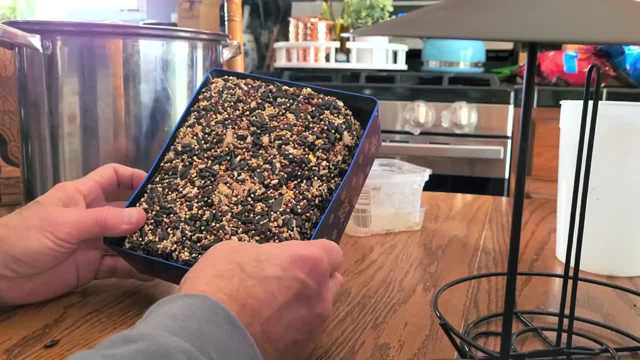 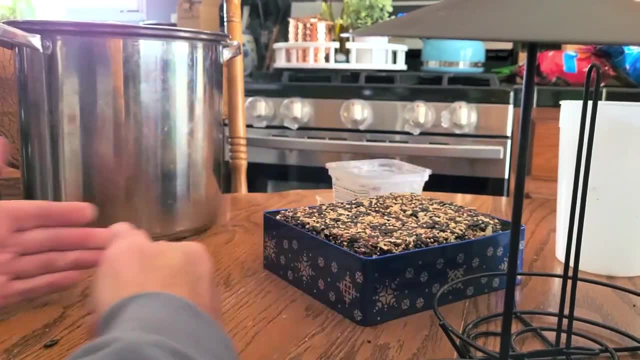 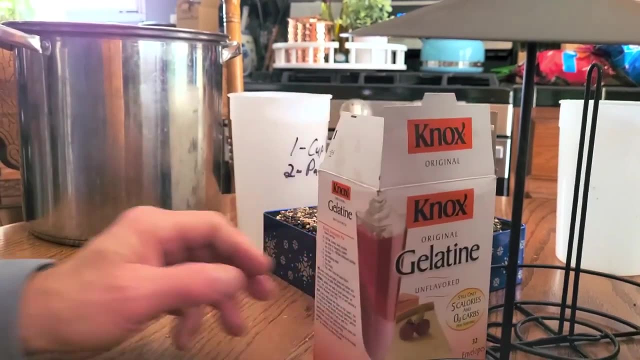 in an Oreo box container that I got for Christmas from one of my kids. So you can make big seed logs like this, which I do have a couple feeders that are this big. You can use any of your mixed seed that you normally use. You can add nuts. Sometimes I add mealworms On this batch. 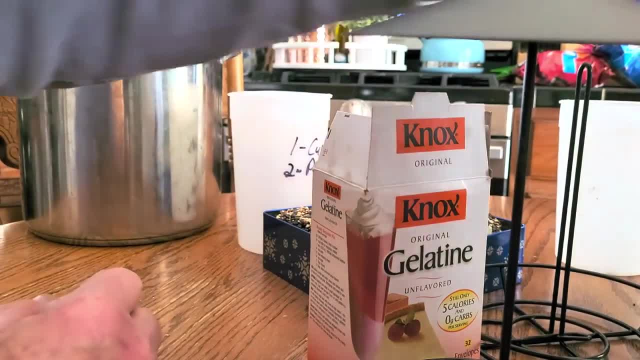 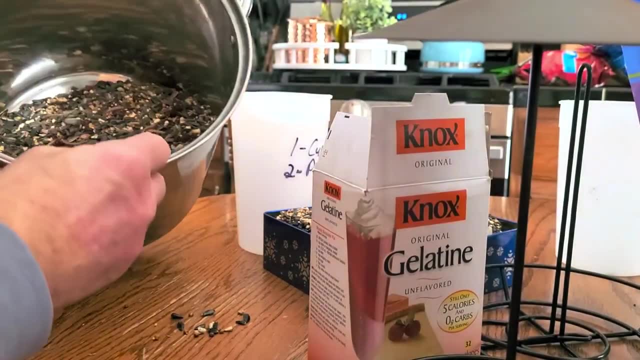 what I'm going to do. I put a quarter cup of mealworms in it and I also put a quarter cup of cranberries. You can put strawberries, cherries, all the birds like those. So I diced up a bunch of cranberries and here's my seed mix. Now I doubled this recipe, so there's actually 10 cups. 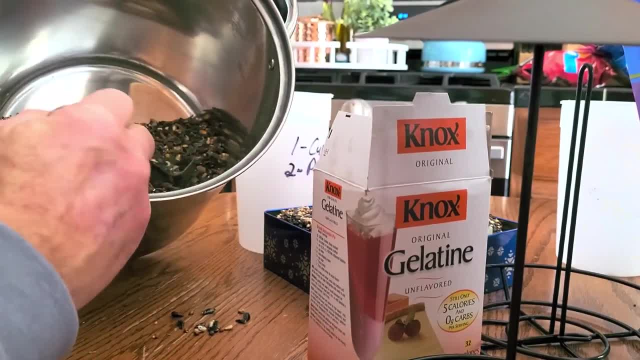 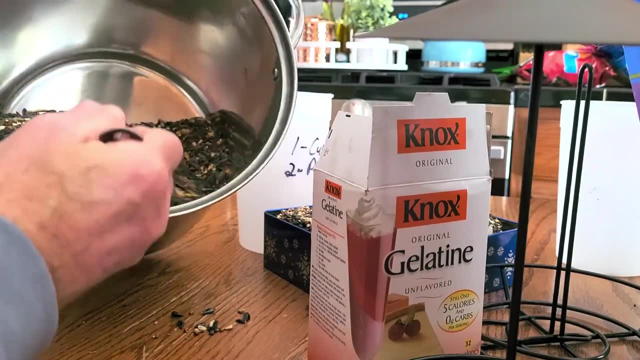 of seed. in here There's nuts, millet, you know, safflower seeds, a little bit of sunflower seeds and, like I said, mealworms and cranberries. So this will be the mix that we use. So I'm going to go ahead and get the water going. 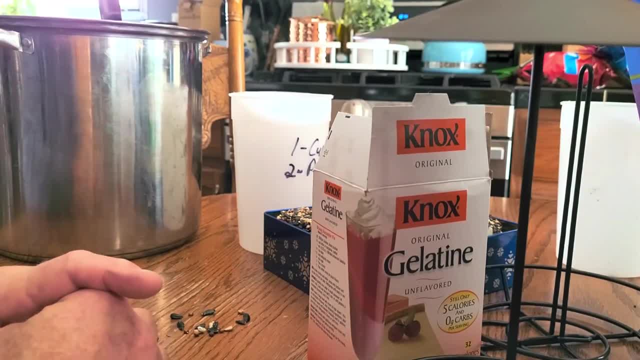 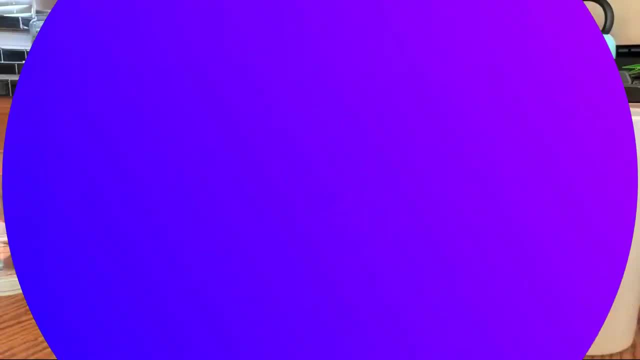 and we're going to dump this gelatin in and stir this up and pour a couple of these and show you what you need to do next. So stay tuned, Be right back. All right, this is Lynn, We're back. Okay, here comes the important part. Now we read that you should. this is: 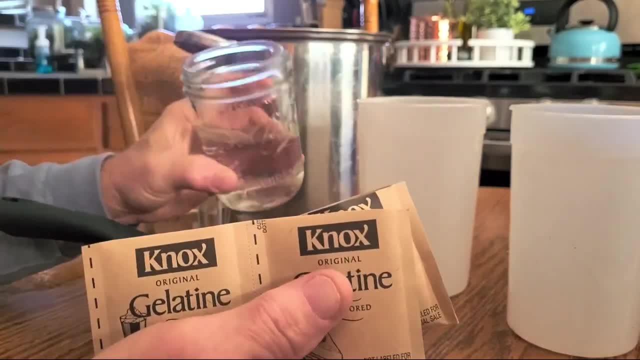 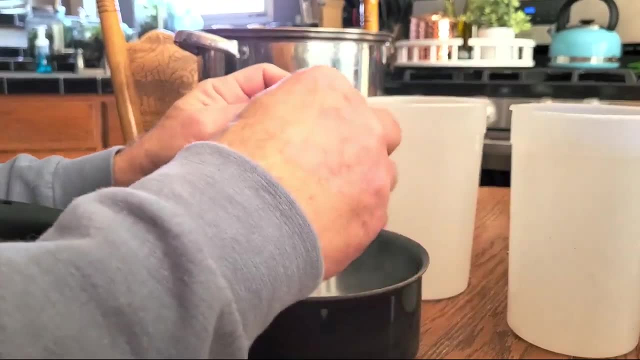 a double recipe, So we're going to use two cups of water. The first cup- this is one cup, 8 ounces- is going to be a cooler water. I'm going to put all four packs of gelatin in here- Kind of dusty. 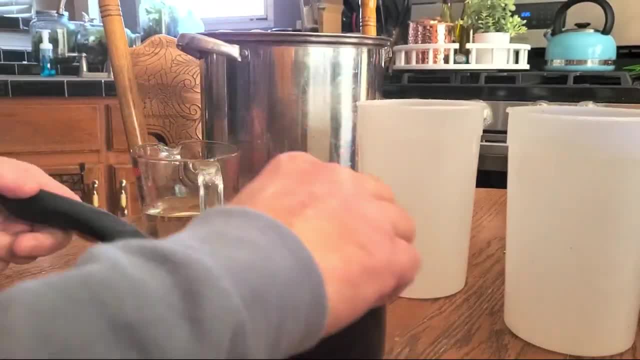 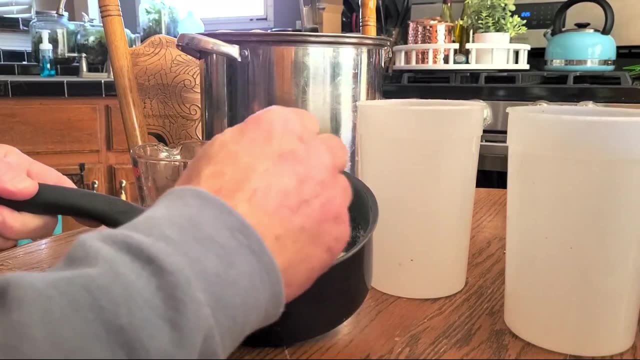 eh, Nox, four packages. What I'm going to do is I'm going to stir this. It's supposed to activate it, So that's kind of a cool liquid. So I'm going to stir this, I'm going to pour. 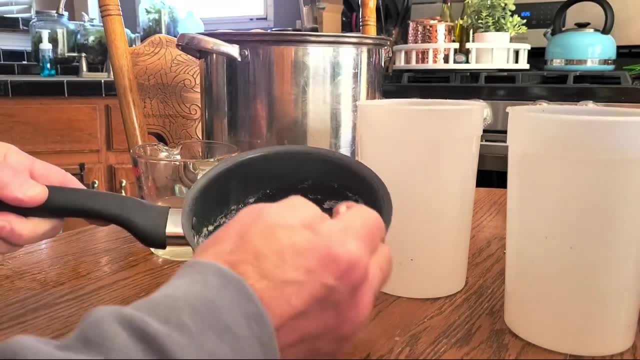 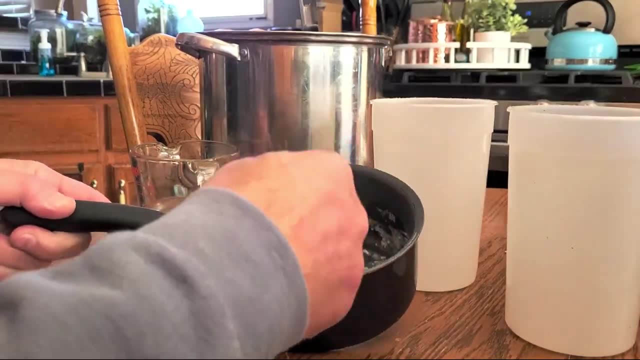 it in. I'm going to stir this. It's kind of clotting right now. It's getting kind of thick. See Kind of cottage cheese really. Next I'm going to add: this is hot tap water. It's not boiled or nothing, It's just warm. 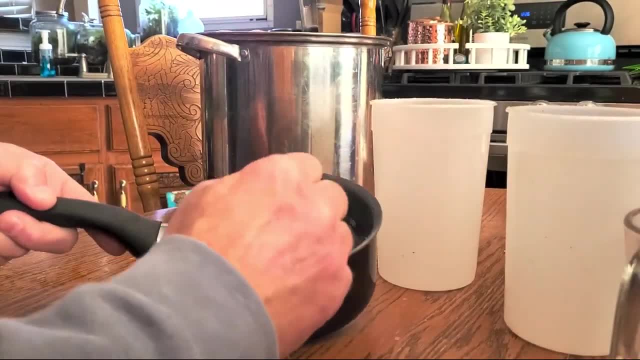 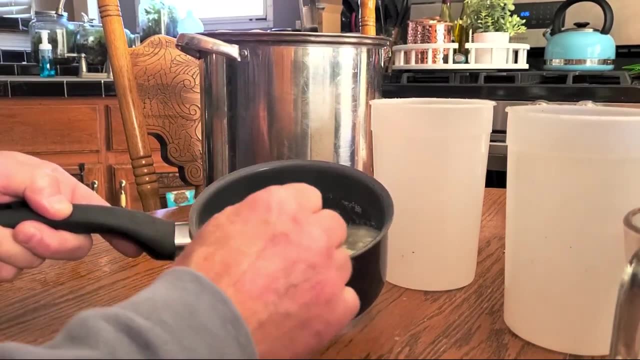 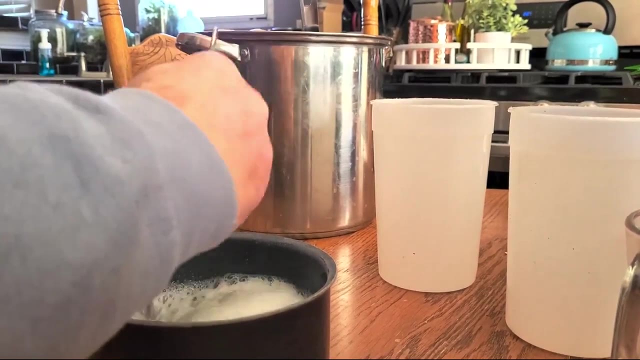 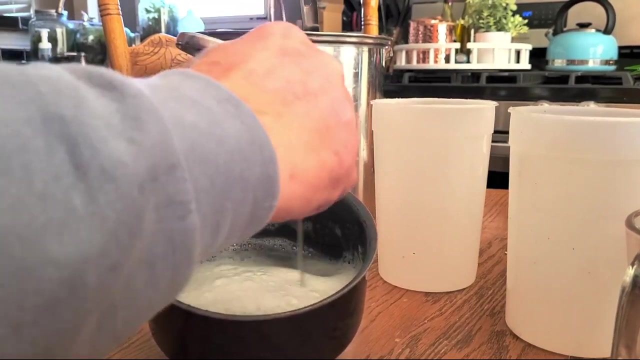 warm, hot tap water. So I'm going to stir all this up. So we got two cups in here of water with four packs of gelatin. We're going to stir this up, Okay, All right. So anyway, I got a whisk and it looks kind of foamy, Kind of like there's dish soap in. 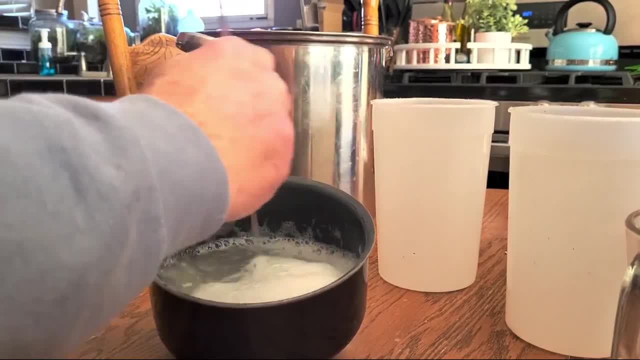 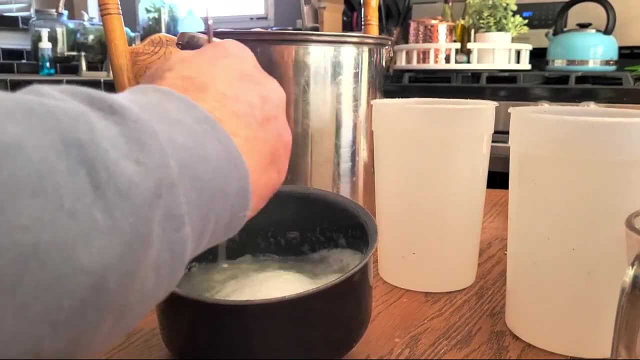 here. but there's not, It's just the gelatin, And then we're going to pour it in our steel canister here and start mixing it into the seed while it's still kind of warm. Okay, Put this aside, I'm going to dump this in. 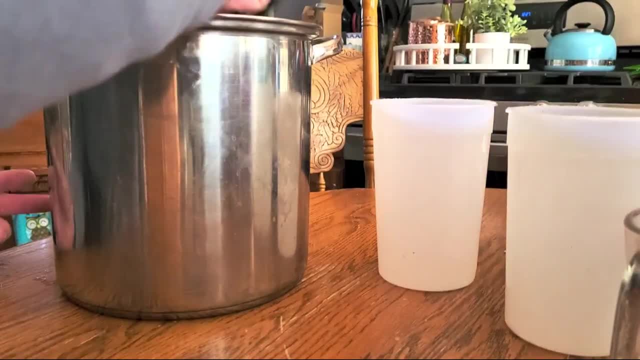 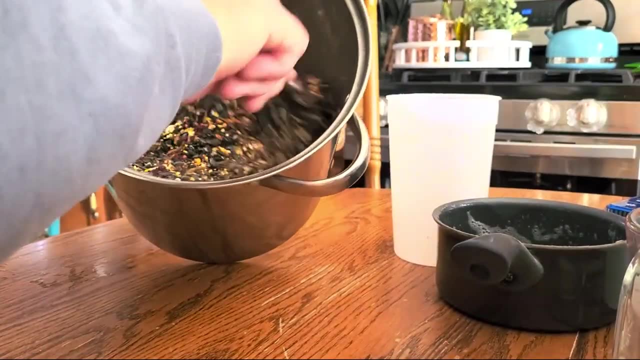 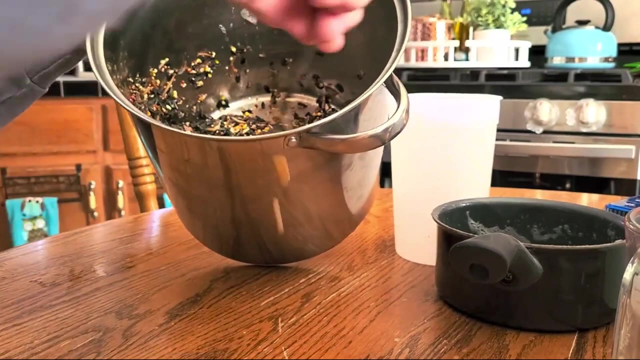 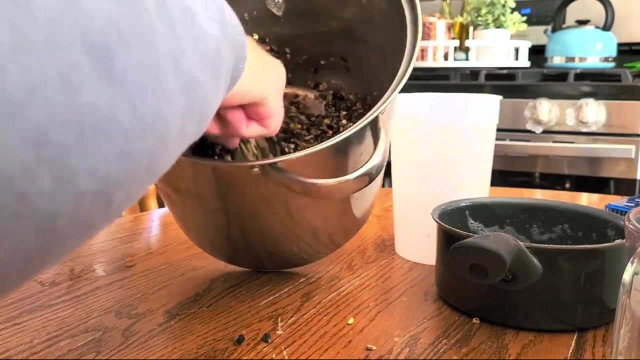 Okay, Our 10 cups of seed while it's still kind of warm. What I'm going to do is I'm going to stir this up so it mixes all this seed in here. And I just got this at Walmart: this kettle, It's like $9 or something. It holds a lot, but when you make lard, it kind of. 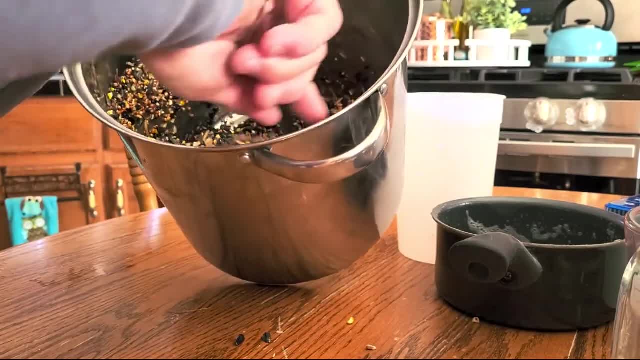 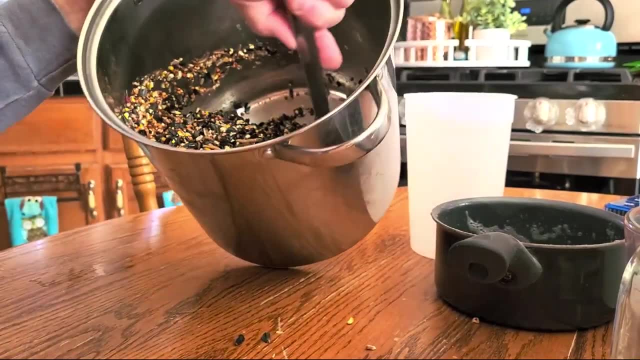 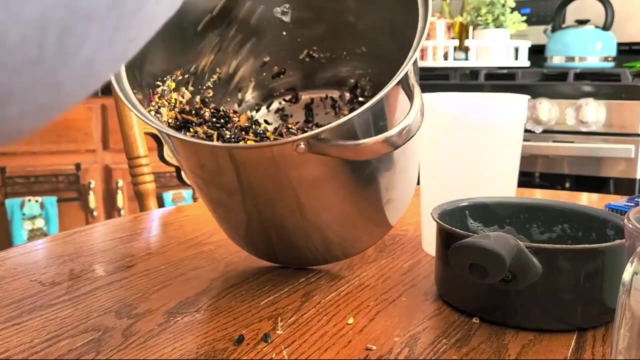 comes in handy. It's easy to clean when you're using greasy lard. So anyway, the seeds are getting wet. I want to make sure you get down at the bottom. Stir this up real good. Everything's kind of mixed. 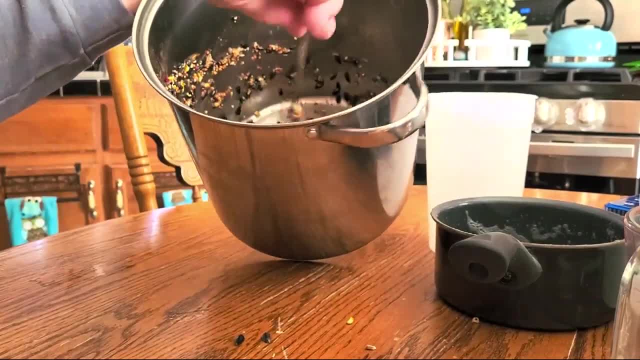 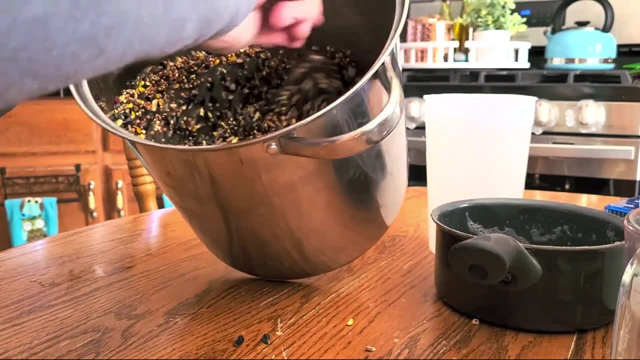 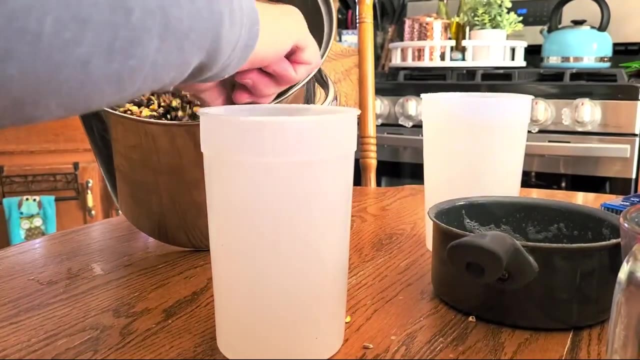 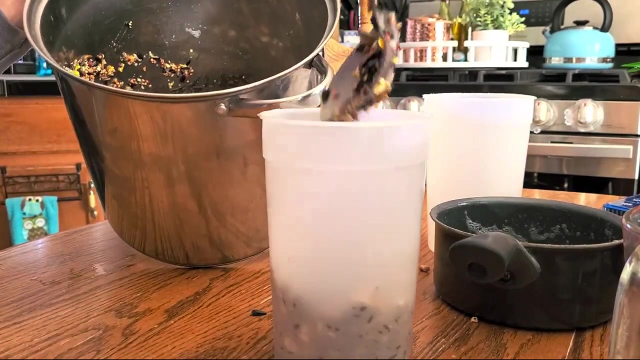 Every little piece in here is nice and wet, Okay, So what we're going to do now is we're going to fill these containers. This all looks like it's pretty consistent. I'm going to fill these up to about- I don't know- a half inch to the top from the top. 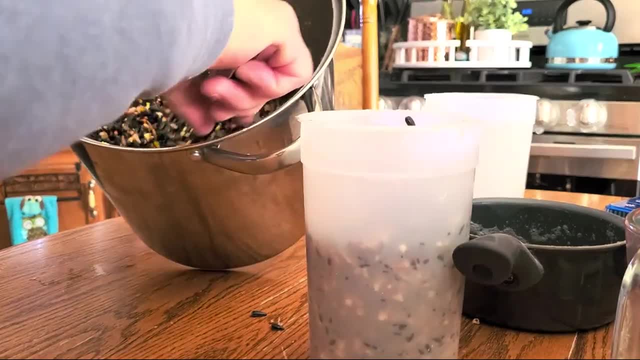 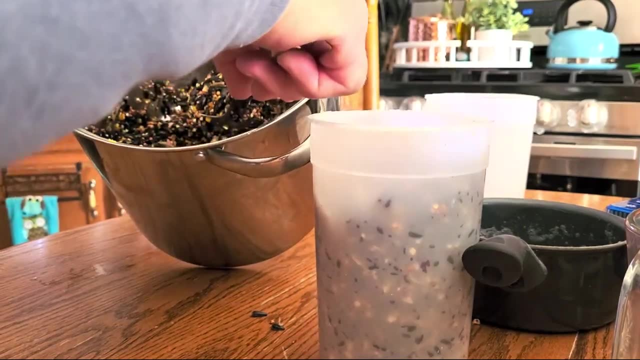 Now the dowel rod that I'm pushing in. it's about a nine-inch dowel rod. It's seven-sixteenths in diameter, But some of the feeders that you buy might only be a quarter-inch rod, So you might have to use a smaller rod. 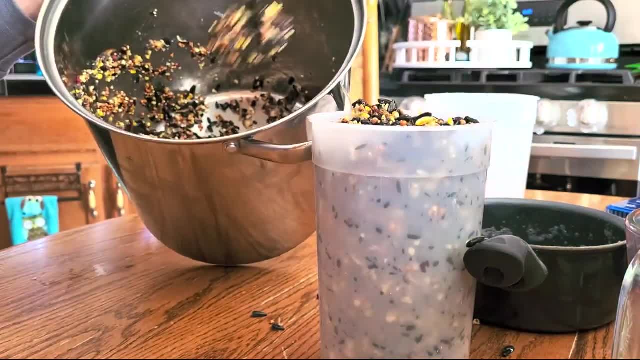 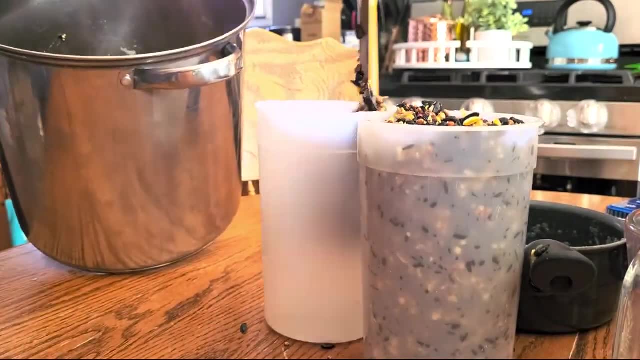 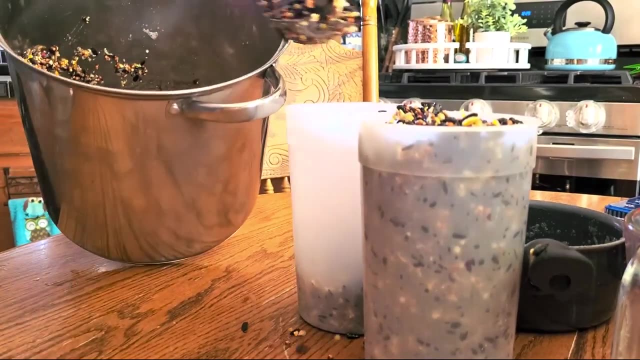 But most of mine are pretty close to a half-inch. So there's one, And if you've got leftover, just put it in another suet container And you can use it. But it should be. it should come out about right. 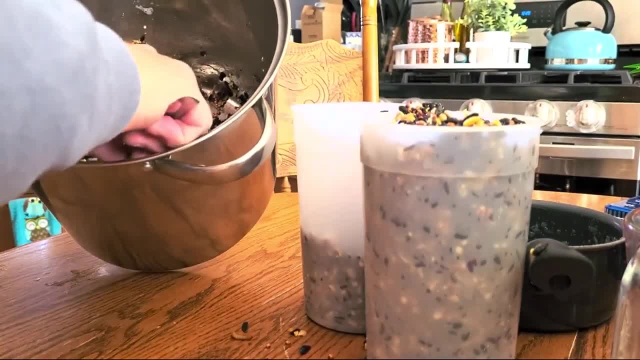 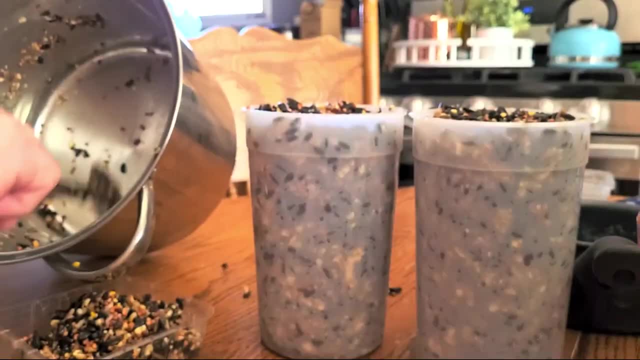 And, yeah, I'm making a mess, Kind of a mess, So we'll get these all spooned in and come back to the next process. And then I did have some extra, But that's all right, We'll save this extra. 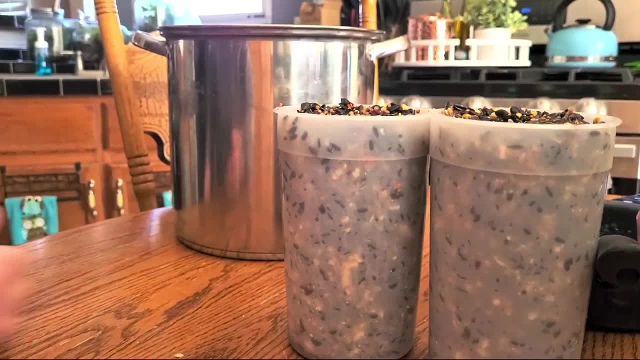 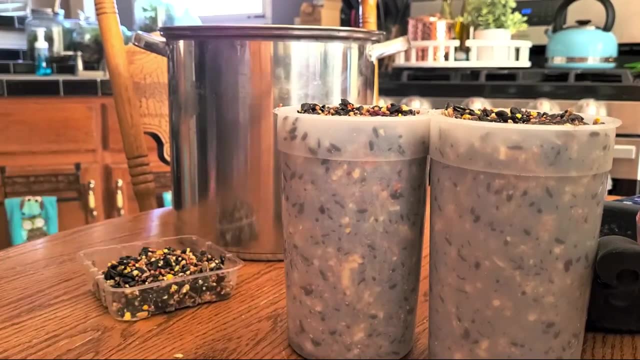 We can use it like in a platform feeder or something later. But you'll get better as you do it. But here's how much I got left over. Okay, now you can find like a can of tomatoes or you can make something out of wood or whatever. 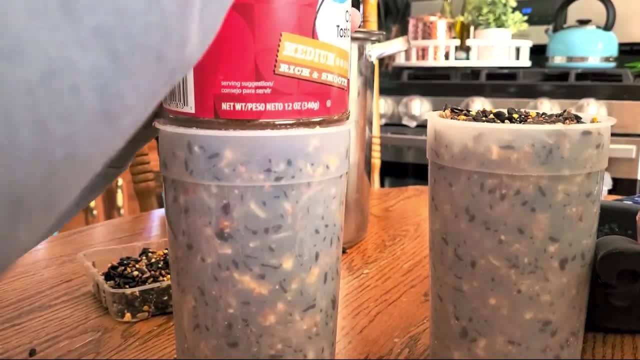 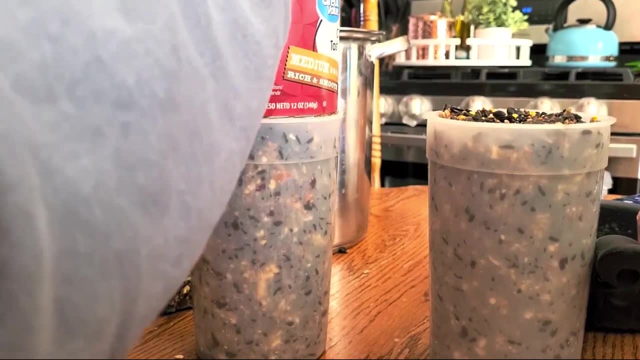 But what you want to do? you don't have a lot of time, But what you're going to do is you're going to smash this down, Compress it. So I'm using just some instant coffee that I drink every morning in the container. 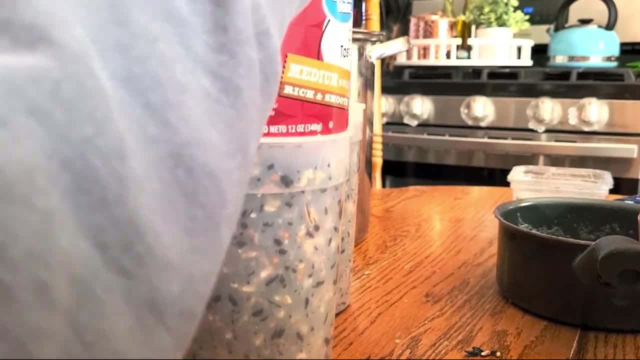 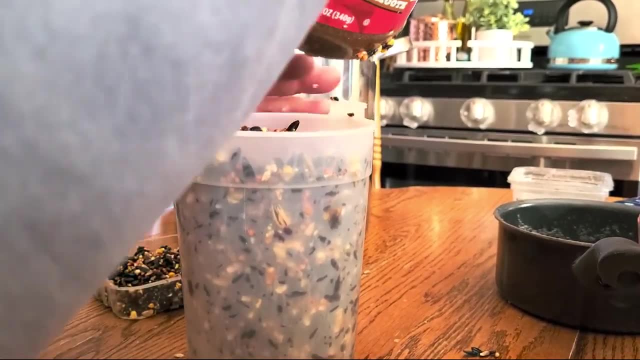 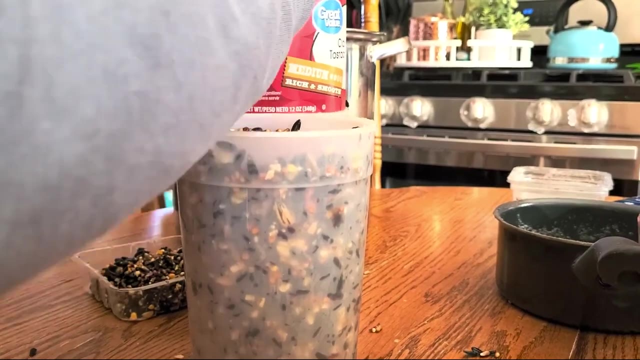 And what I'm doing is I am pushing pretty hard, compacting all that together so it'll stick. It's all right if you still have some loose seeds on top and stuff, So those are pushed down pretty good. I'm using all my weight into it. 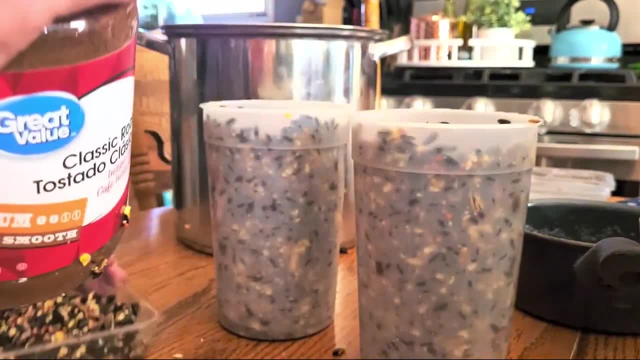 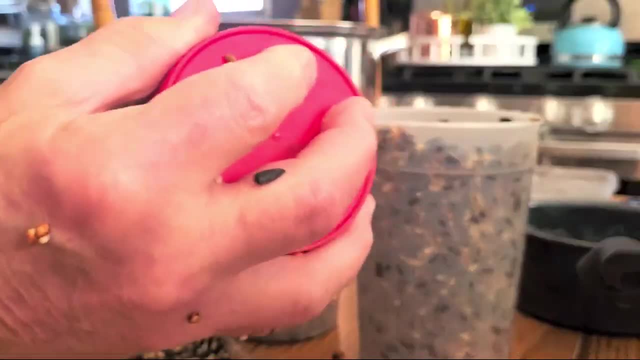 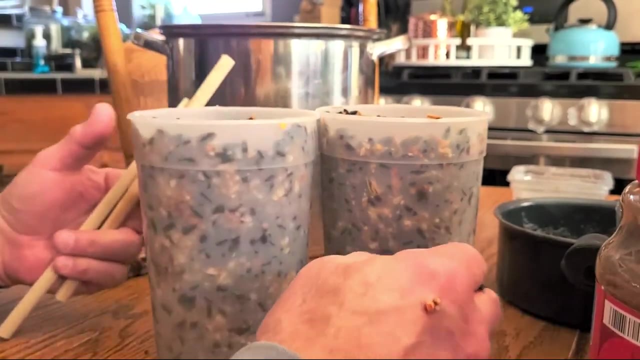 So those are pushed down, And I'm going to do this little one also, So those look good. Now here's what I did. I cut dowel rod. This is 7- 16 dowel rod, which is big enough for the feeders that I use or if I want to put a string through it. 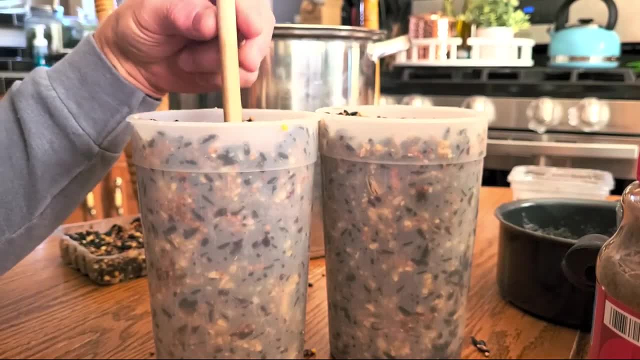 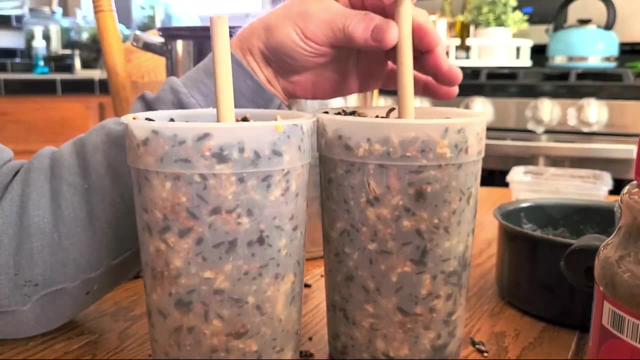 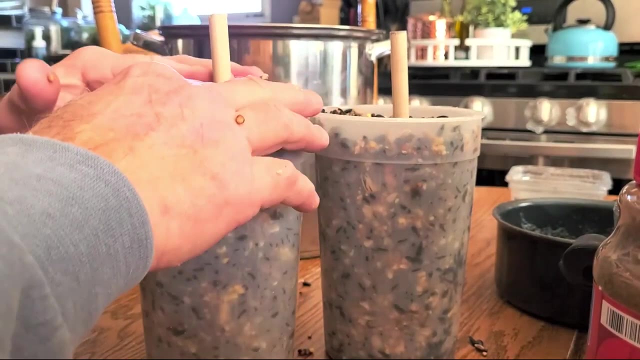 So I just go right in the center And I go right down through the bottom of it So I hit the plastic. I'm going to do both of those right now. So I hit the bottom And I'm going to kind of make sure they're level. 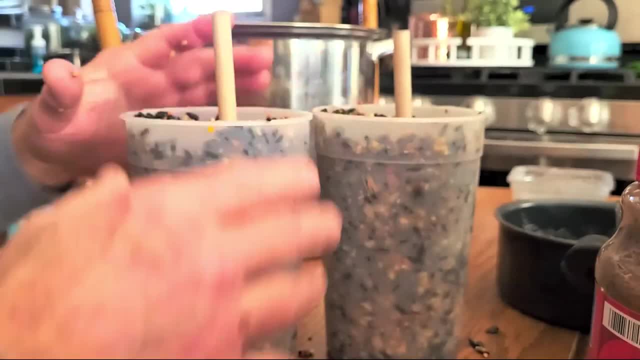 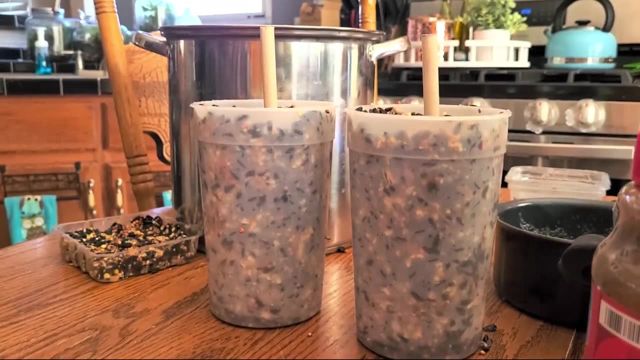 Push some of the seed down with my fingers. So that's what it looks like right there. okay, Now what you'll want to do next, very, very important: You want to put both of these in the refrigerator for one hour. 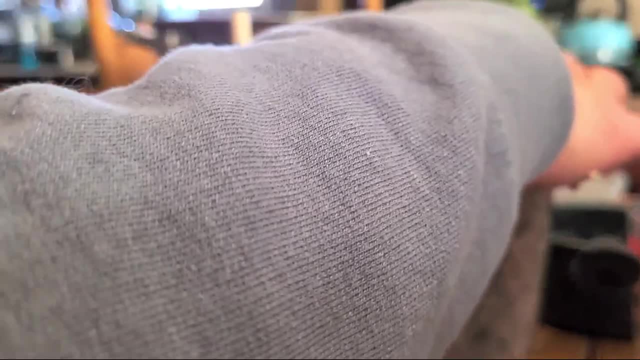 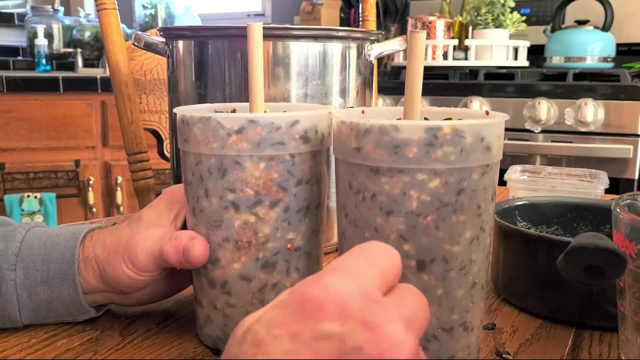 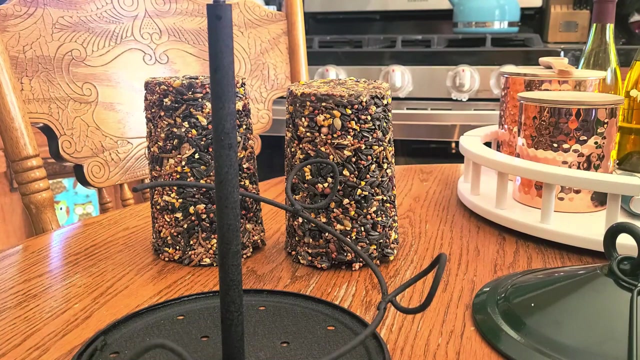 Let them set. They'll set up like jello. You know it'll end up getting hard, So put them in there for an hour And then we're going to finish this up. I left the two seed cakes in the refrigerator for a couple hours yesterday. 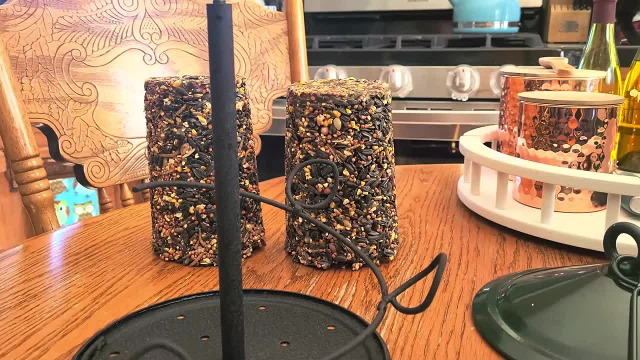 And then I took them out And I just left them out in the open air to dry. They're pretty dry. You can also freeze these if you want. Now come summertime, I don't know how long these will last. I really don't know.